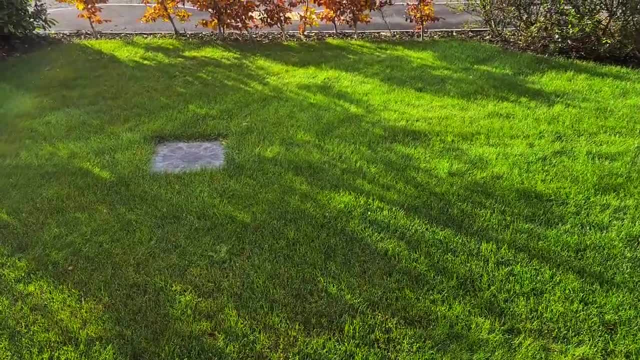 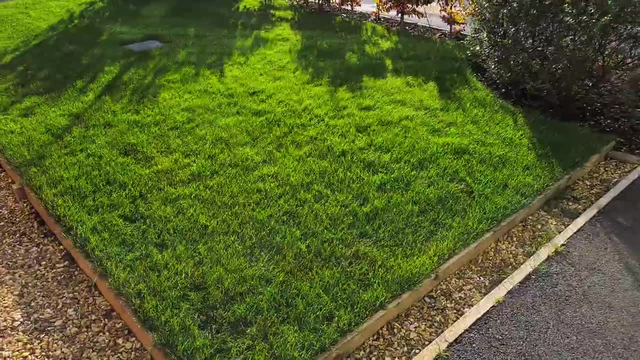 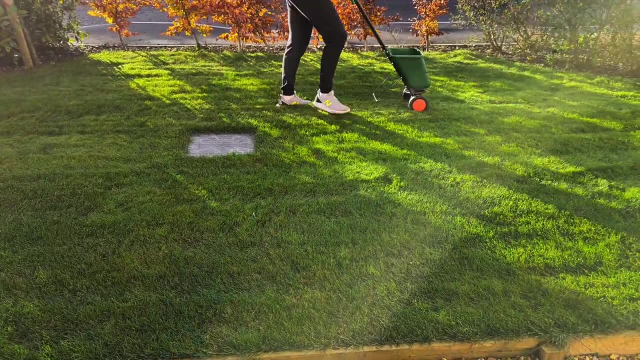 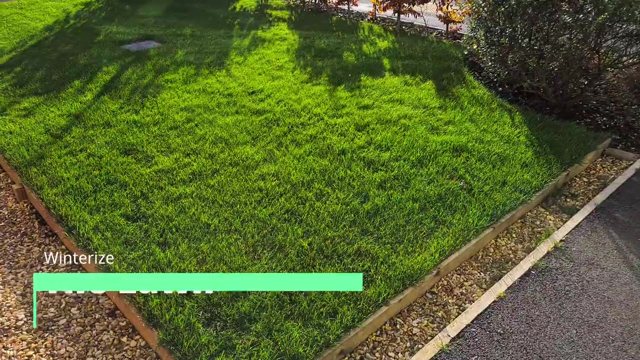 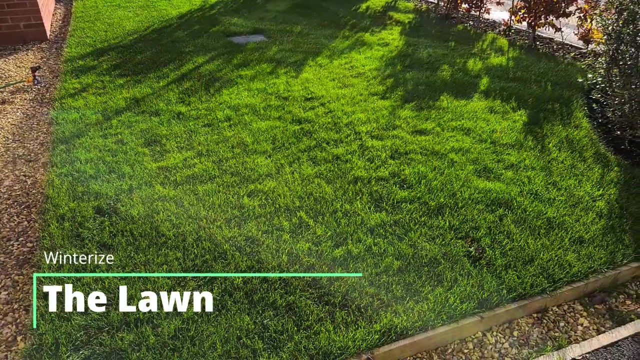 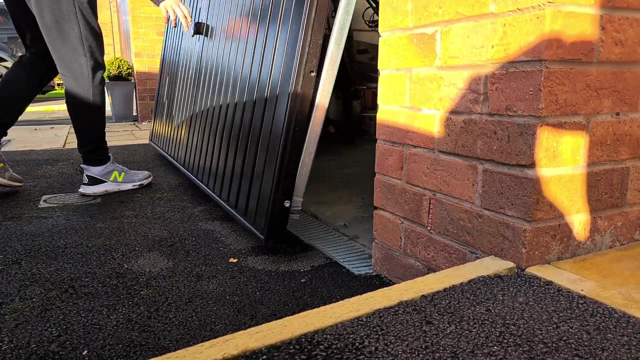 Here's a secret to keep a deep, dark green throughout the winter months: in less than five minutes. Keeping a dark green lawn over the winter months can be a real challenge. This is because the light starts to reduce, the rain starts to increase and the grass also goes into dormancy and isn't grown as vigorously. 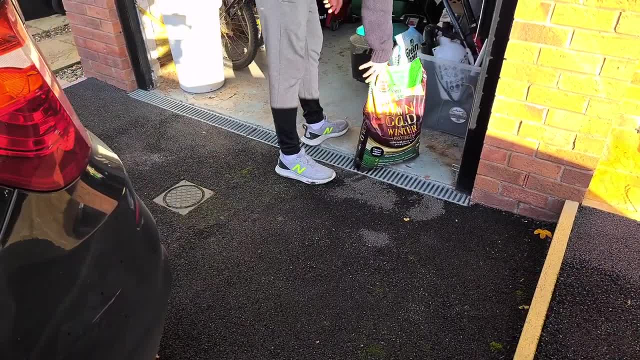 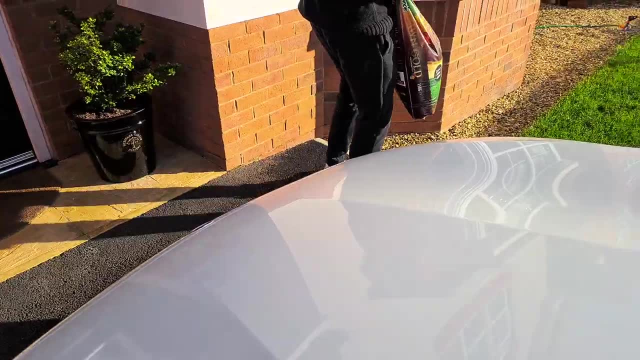 In this video, we're going to be looking at something you can apply to your lawn in order to keep that dark green look and also combat moss. I'm going to be doing the last cut of the season. It's mid-November- right now. 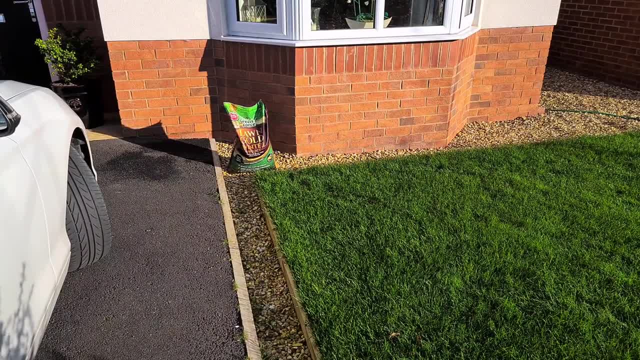 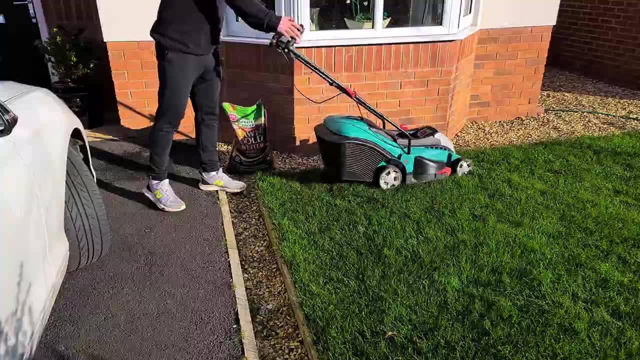 and the grass growth is really starting to slow down. This is a product that I'm going to be using for the winter months. This is a product that I'm going to be looking to apply after the last cut of the season. It's a slow-release formula that's going to help drag me through the winter months. 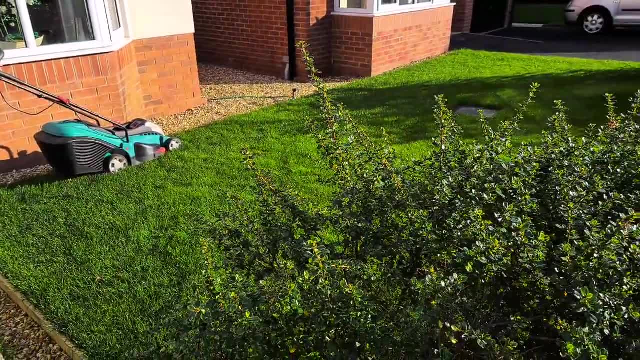 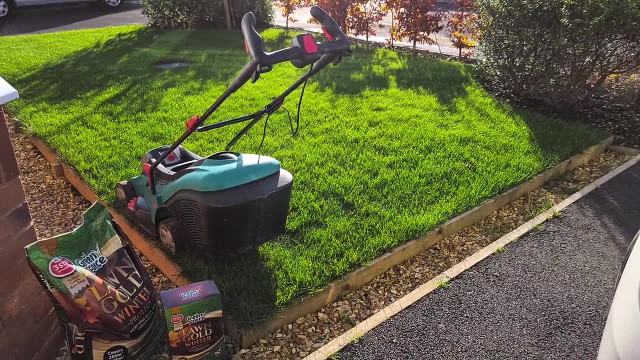 and keep a green appearance on the lawn First up. I'm going to take a look at what I might need in order to apply this treatment. First of all, I'm going to take the lawnmower. I'm going to raise this up, set it on a high setting. 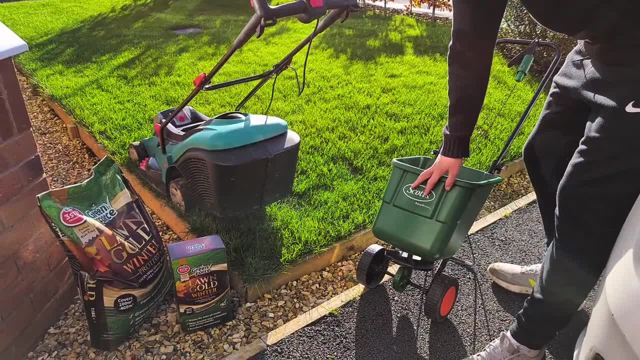 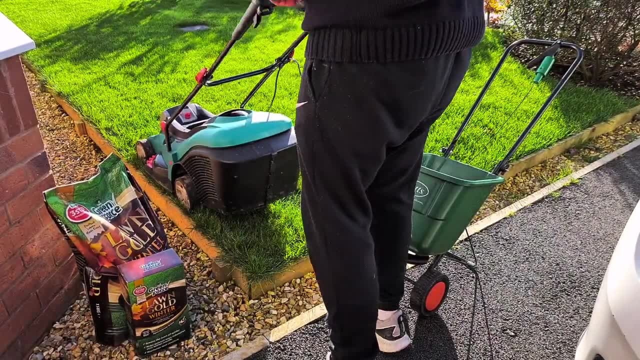 I don't want to cut the grass too short so it can get plenty of light and continue to photosynthesize. I've got the product that I'm going to be using, which is called Lawn Gold Winter Protect, and also my Scotts Rotary Spreader. 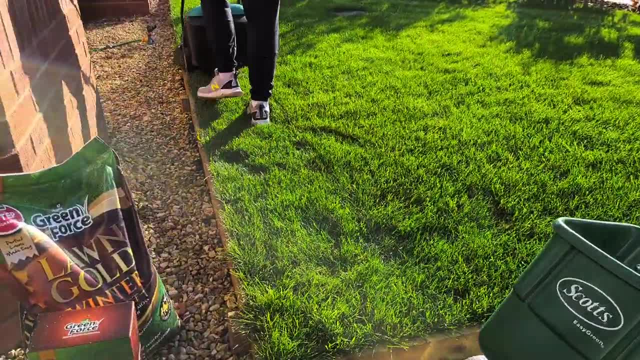 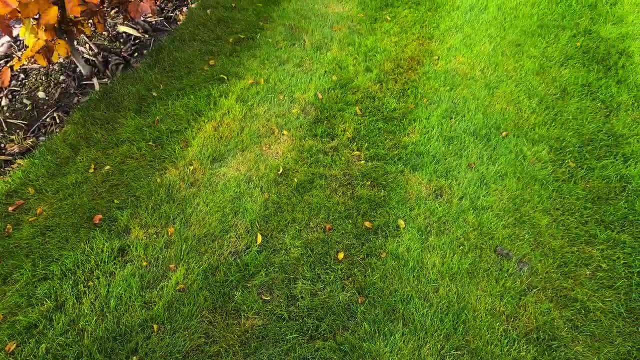 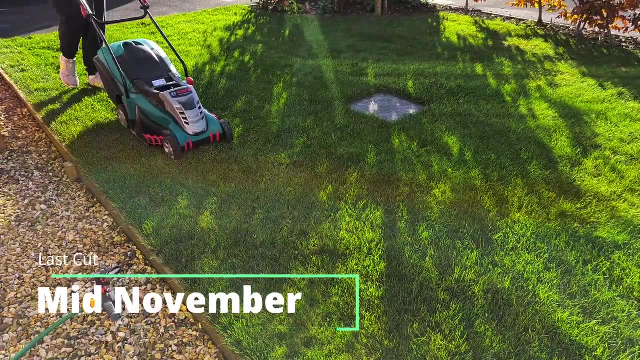 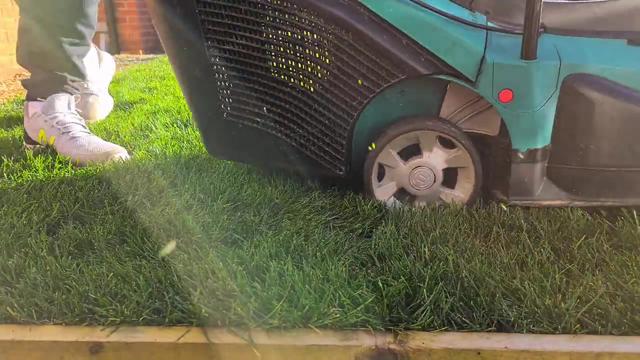 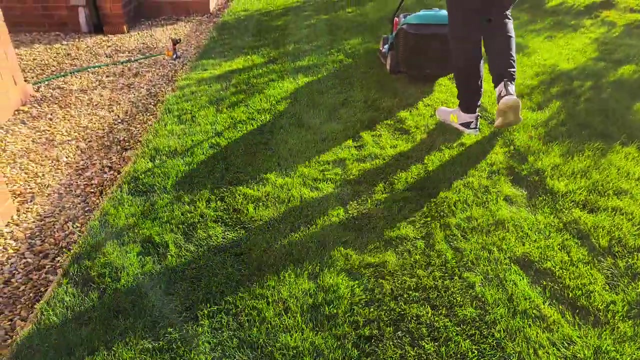 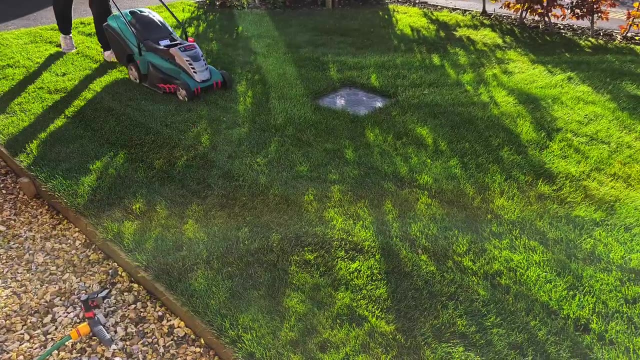 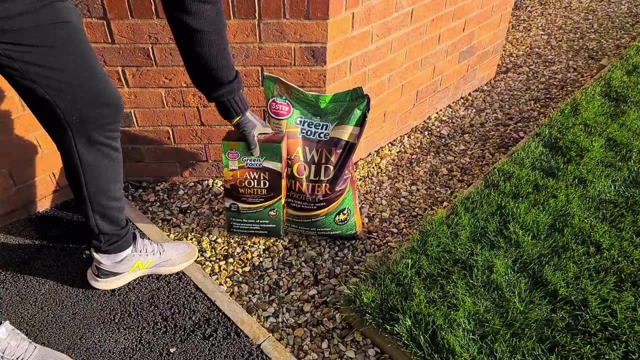 Coming up. I'm going to be going through some of the contents of this particular product, but first let's give the lawn the last cut of the year, pick up the leaves and get it ready for treatment. ✌️, ✌️, ✌️. 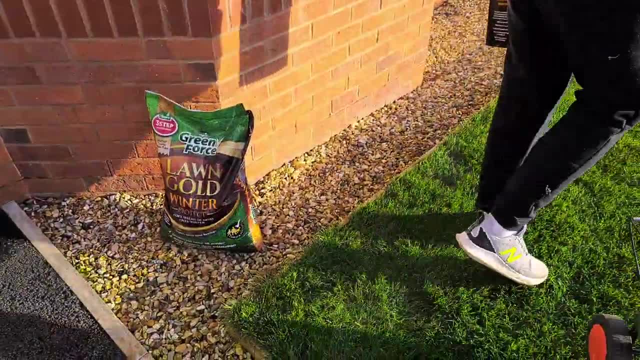 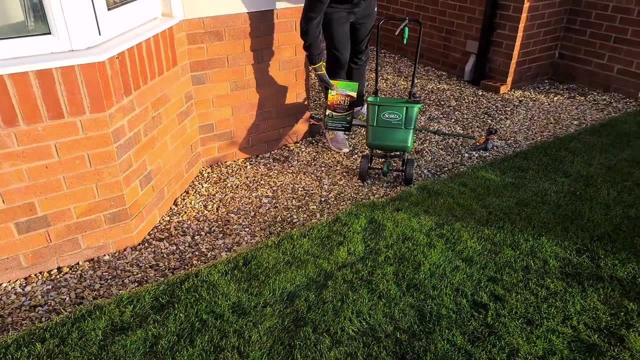 Now the lawn has been trimmed back, I'm going to look at the lawnmower for treatment. ✌️, ✌️, ✌️ at applying the lawn gold winter protect. this product contains a slow release iron and if anybody's used iron before, you'll know that it will stain hard surfaces. and it's also good. 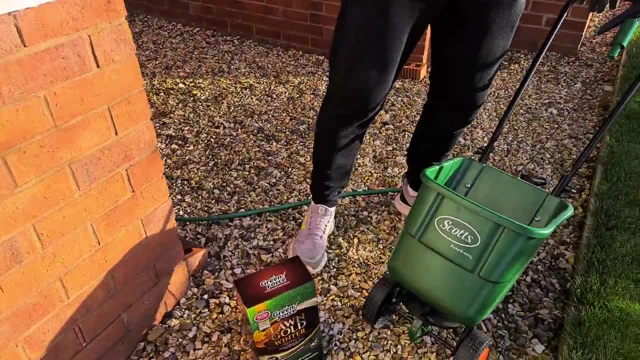 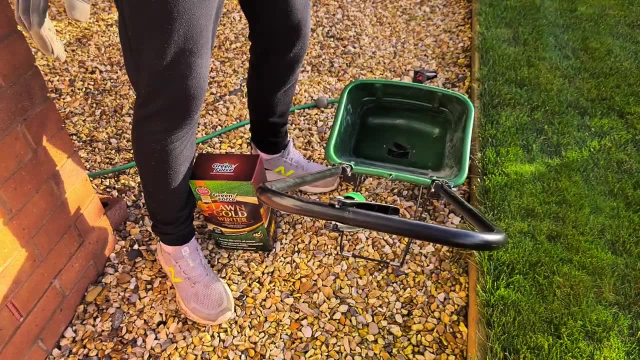 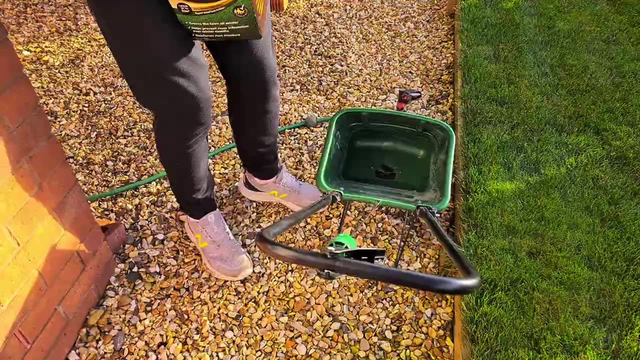 practice to transfer any chemicals or products that you're applying to the lawn off the lawn in case you spill any and it can damage the lawn. so here i've just stepped into this little bit of a side area. i've set my spreader on around a 27- 28, setting this particular box of lawn gold winter. 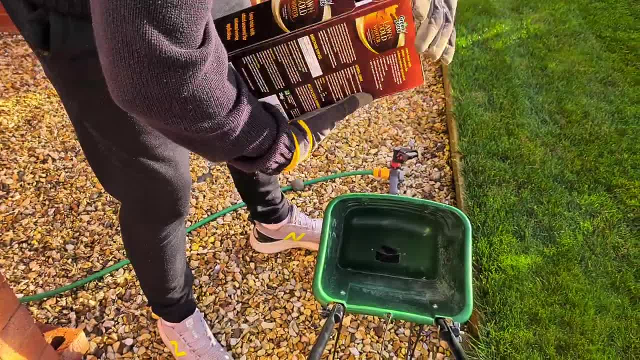 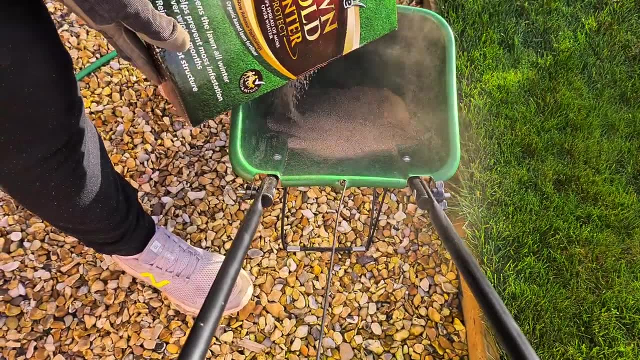 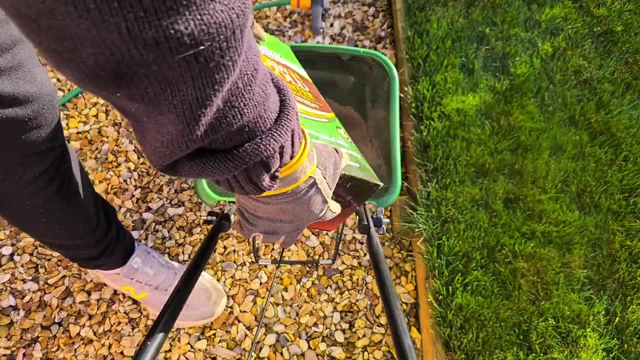 protect can cover up to 80 square meters. my area is around half of that, so i'm going to use roughly half a pack. you can do this by punching a little hole in the side of the pack and transferring what's left into the spreader. i always like to use gloves when handling any form. 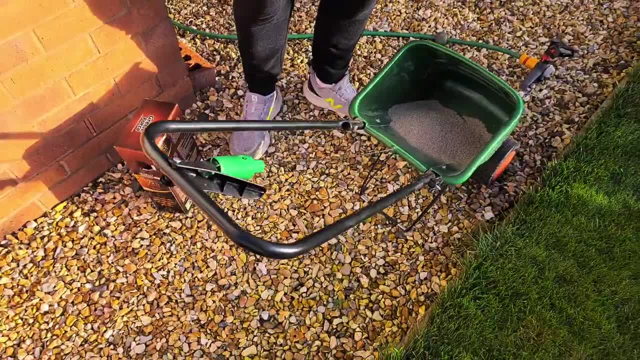 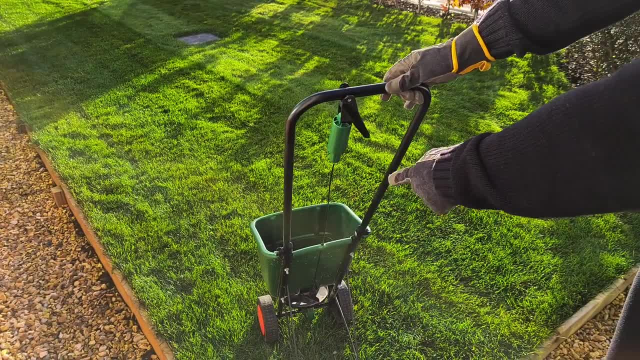 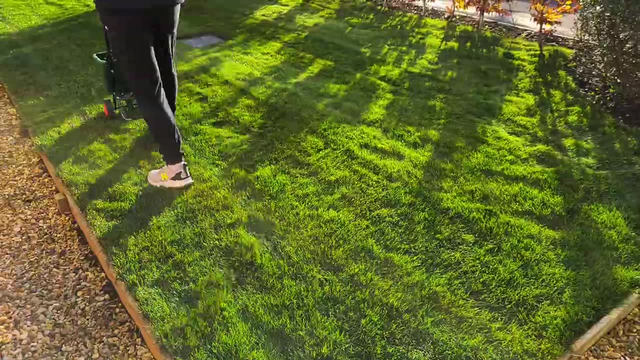 of chemical products like this, just for best practice and health and safety. but all the advice can be found on the box and please read the label, one of the things that i thought i'd share a little tip with you about this spreader: is you actually want to pull the trigger after? 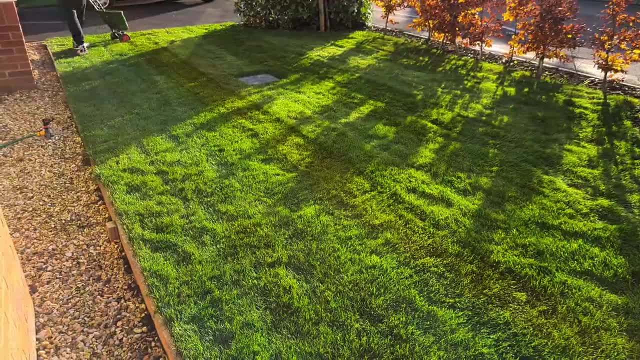 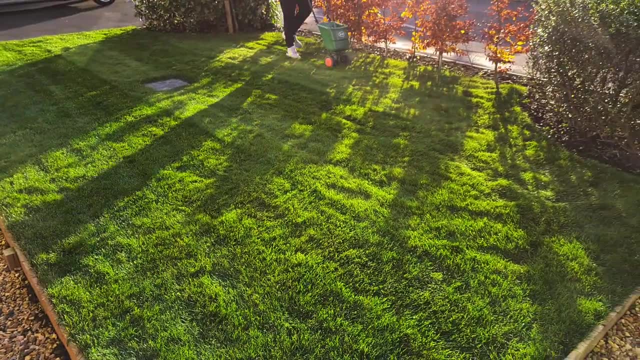 you've started moving. if you pull the trigger first and then start moving, you can get a bit of a clump or excess residue left at the start. so start moving, pull the trigger and then run the edge and pass around your lawn if you're looking to buy any of these products. 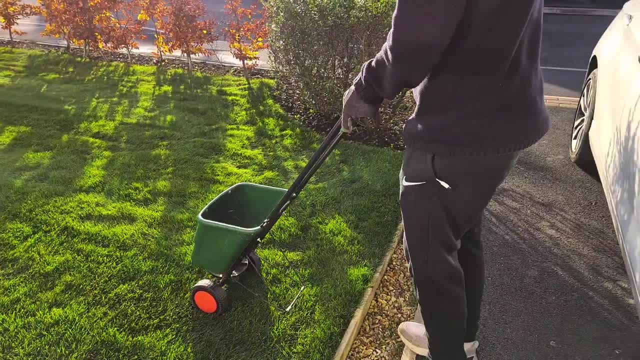 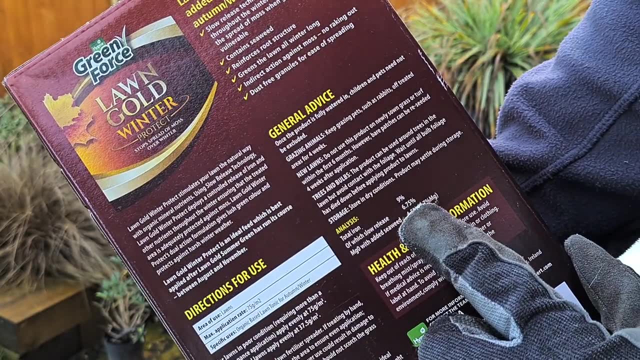 you can find a link to them in the description below, and let's take a little look about what's inside the box. so overall you've got a total iron of nine percent, with nearly seven percent of that being slow release, and on top of it you've got 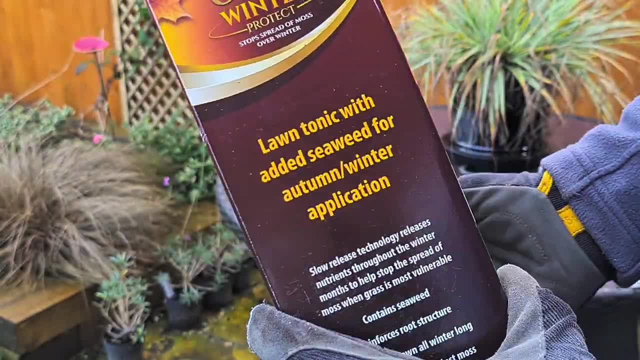 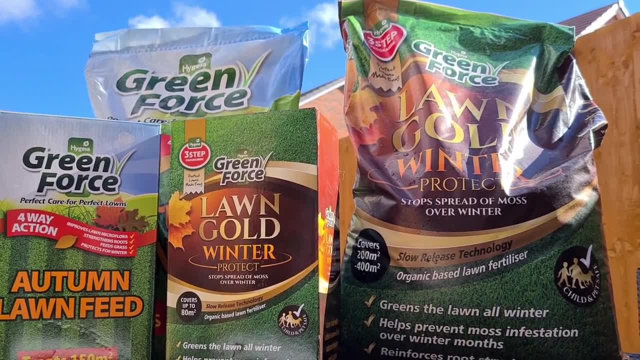 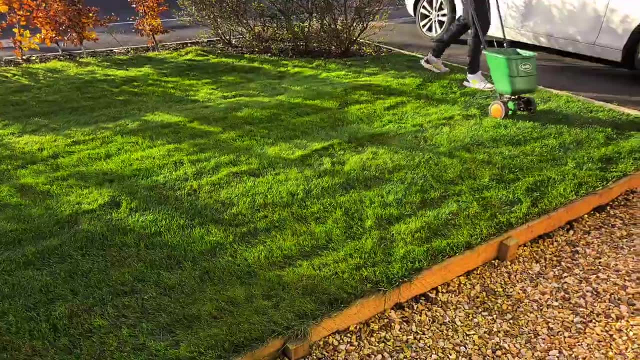 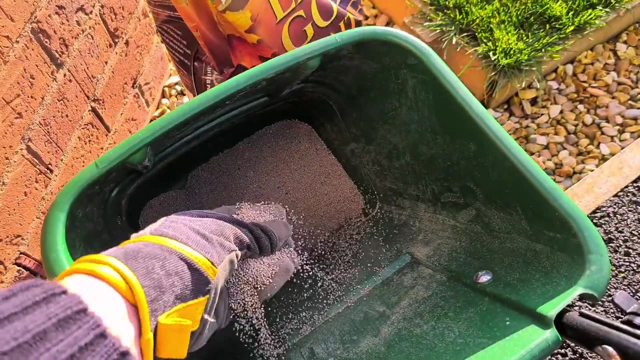 and the sun and the sun and didn't create moisture outside, so definitely use a rearrangement and a few bites in between such products. the pellet size for this product is actually quite small and personally i found it spread really well, evenly and finely across the lawn. i'm hoping to see some results in the coming days after this. 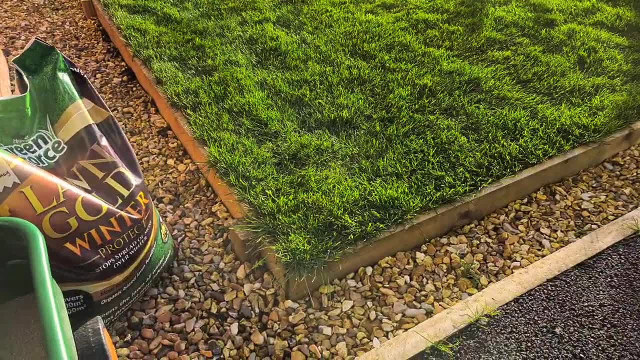 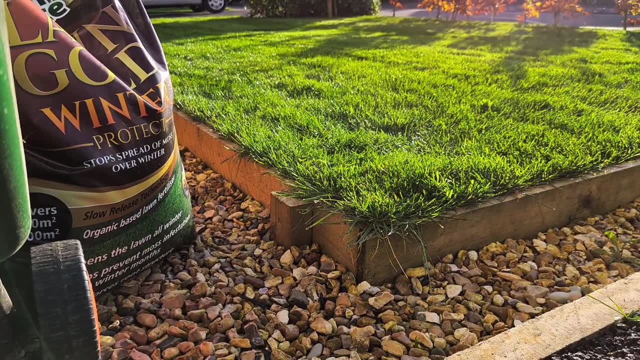 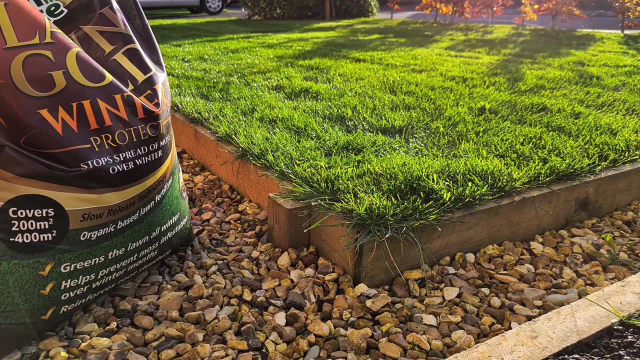 product gets washed in and maintained a nice green lawn throughout the winter. You will see just in the bottom of the shot there in the pass where I've spilt iron products onto the hard surfaces. so if you do spill any, make sure to wash or hose down the surfaces that you get it on, just to prevent any of this orange staining you might. 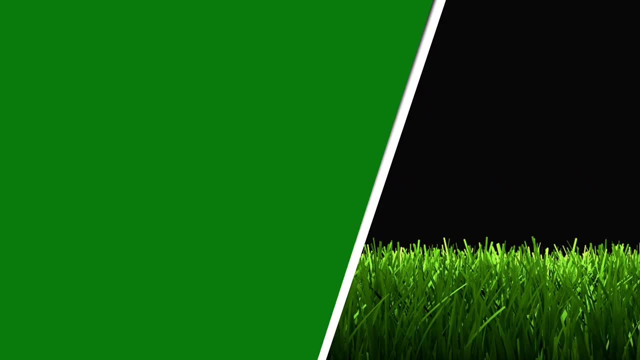 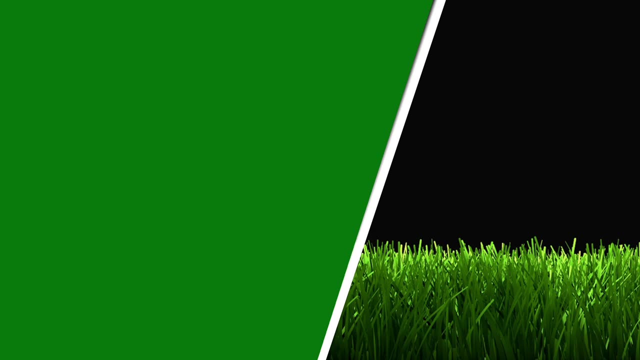 see. If you enjoy lawn care videos and winter lawn care, please consider subscribing to my channel and checking out some of the other videos that I've made. Thanks for watching. 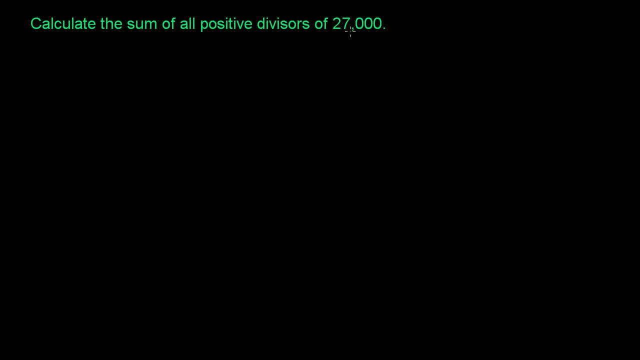 Calculate the sum of all positive divisors of 27,000.. The easiest thing that I can think of doing is first take the prime factorization of 27,000, and then that'll help us kind of structure our thought of what all of the 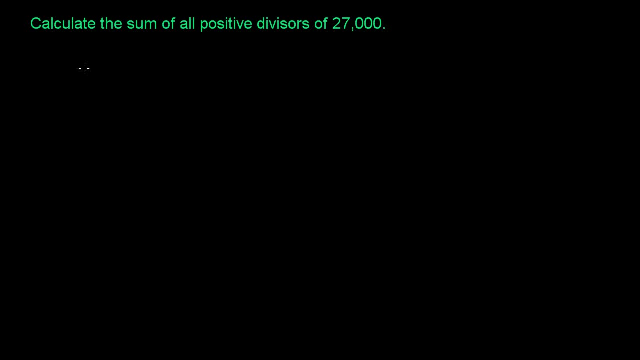 different divisors of 27,000 would have to look like. So 27,000 is the same thing as 27 times 1,000, which is the same thing as 3 to the third times 10 to the third, And 10 is of course the same thing as 2 times 5.. 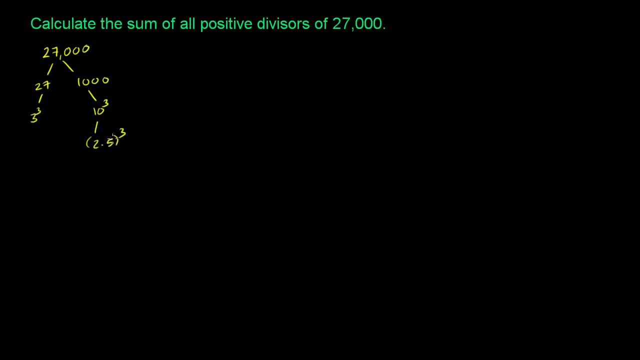 So this is the same thing as 2 times 5 to the third, or it's the same thing as 2 to the third times 5 to the third. So 27,000 is equal to 2 to the third times 3 to the third. 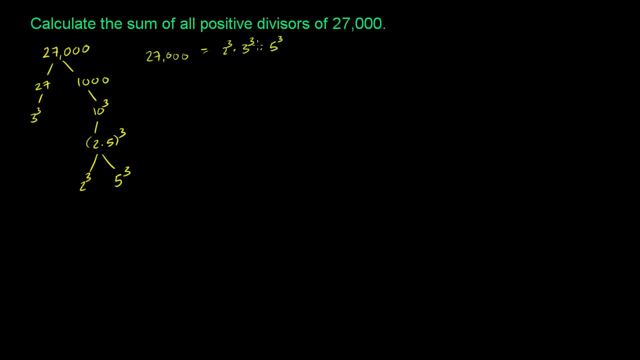 times 5 to the third. So any divisor of 27,000 is going to have to be made up of the product of up to three 2's, up to three 3's and up to three 5's. So let's try to look at all the combinations and think of.